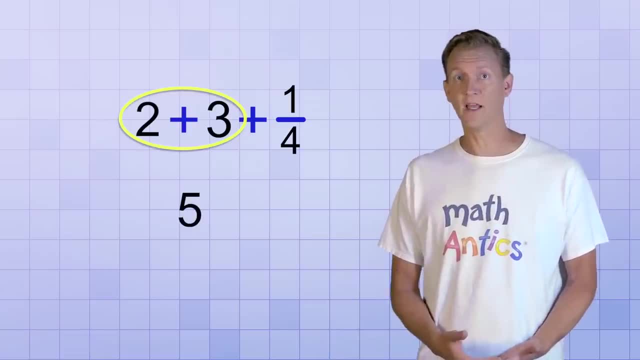 Well, that's easy. All you have to do is add the 2 and the 3 to get 5, and you'll have 5 plus 1 fourth, which is the mixed number 5 and 1 fourth. 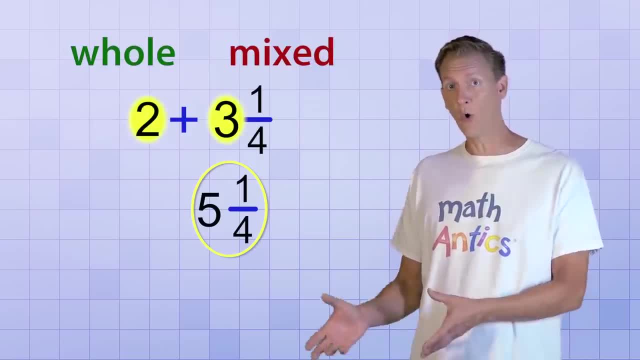 So if you need to add a whole number to a mixed number, you can just add the whole number parts and you're done. 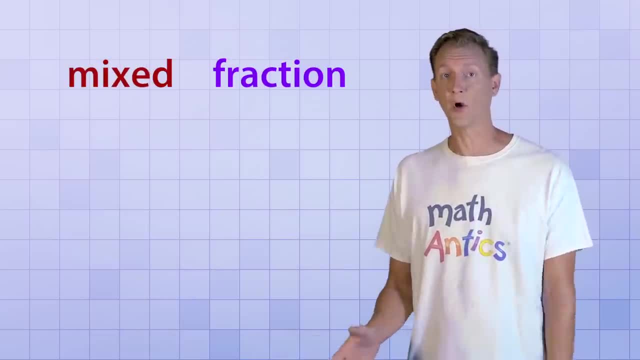 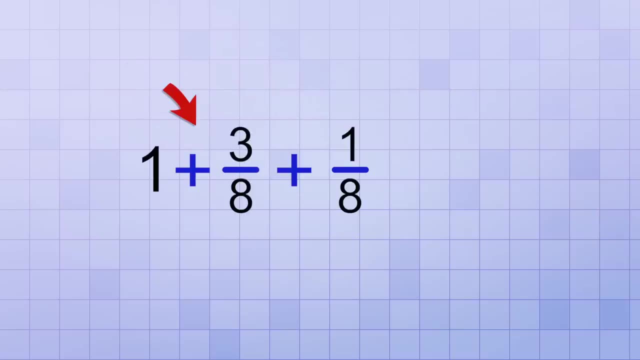 OK, but what if you need to add a mixed number to a fraction, like in the problem 1 and 3 eighths plus 1 eighth? Again, if you remember that 1 and 3 eighths means 1 plus 3 eighths, then you can see that this problem is really 1 plus 3 eighths plus 1 eighth. That looks pretty easy also! 3 eighths and 1 eighth are what we call like fractions. They have the same denominator and can be added easily. 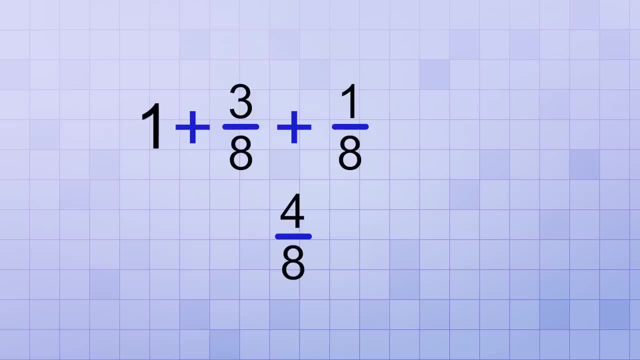 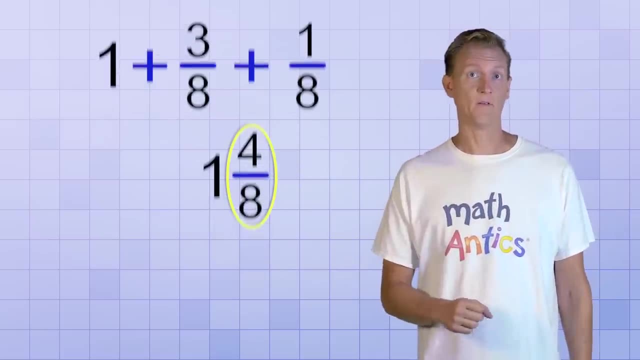 3 eighths plus 1 eighth equals 4 eighths. So our answer is simply the mixed number 1 and 4 eighths. Oh, but you might notice the fraction part can be simplified. 4 eighths simplifies to 1 half, so we should write our answer as 1 and 1 half instead. 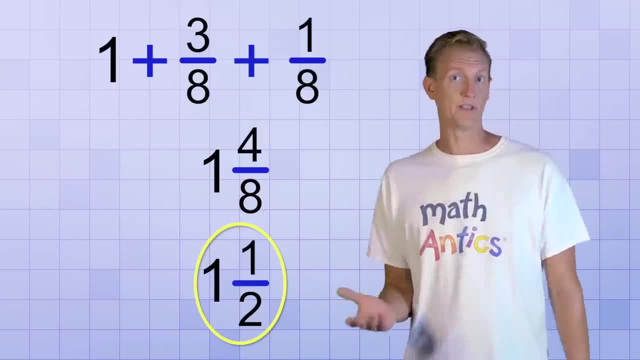 It's not mathematically wrong if you don't simplify a fraction, but teachers and tests usually require you to simplify whenever you can, so it's a good habit to get into. 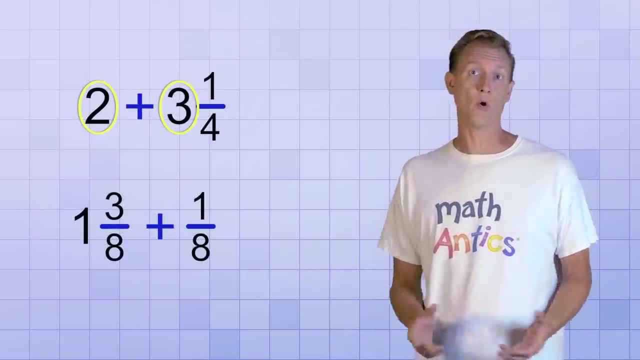 Notice that in each of those examples, we just added whole numbers to whole numbers and fractions to fractions. 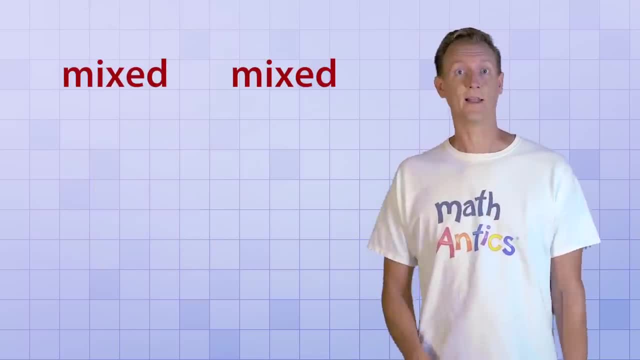 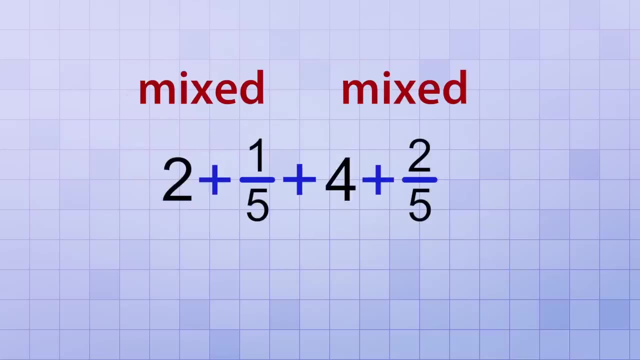 And it works the same way when adding a mixed number to a mixed number, like 2 and 1 fifth plus 4 and 2 fifths. Again, let's show our mixed numbers with the plus signs so we can see the real problem. 2 plus 1 fifth plus 4 plus 2 fifths. Because all of these parts are being added and addition has the commutative property, it really doesn't matter what order we do the addition in. That means we can rearrange it. We can change this problem to make it simpler. Now we have 2 plus 4 plus 1 fifth plus 2 fifths. Adding the whole numbers is easy. 2 plus 4 equals 6. And adding these like fractions is easy too. 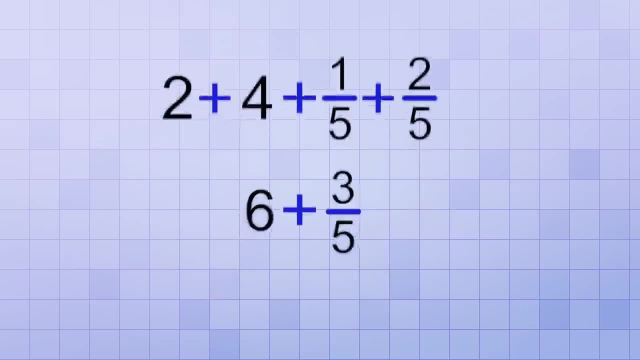 1 fifth plus 2 fifths equals 3 fifths. That leaves us with 6 plus 3 fifths, which is the mixed number 6 and 3 fifths. 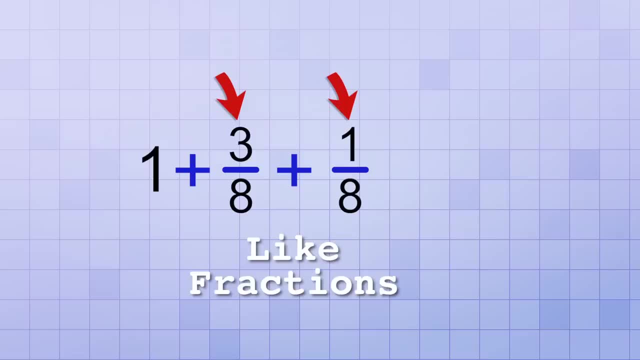 3 eighths and 1 eighth are what we call like fractions. They have the same denominator and can be added easily. 3 eighths plus 1 eighth equals 4 eighths, So our answer is simply the mixed number 1 and 4 eighths. 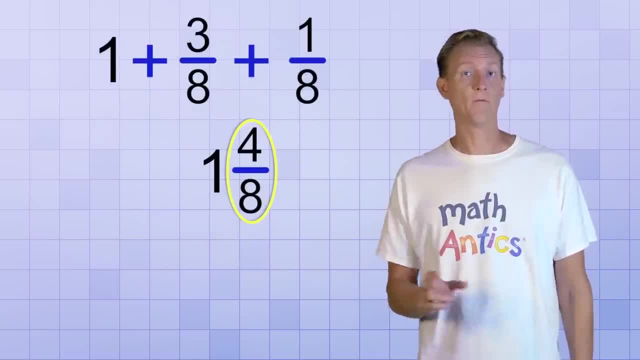 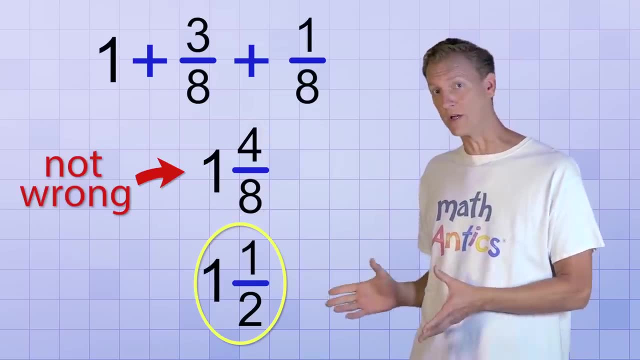 Oh, but you might notice the fraction part can be simplified. 4 eighths simplifies to 1 half, so we should write our answer as 1 and 1 half instead. It's not mathematically wrong if you don't simplify a fraction. 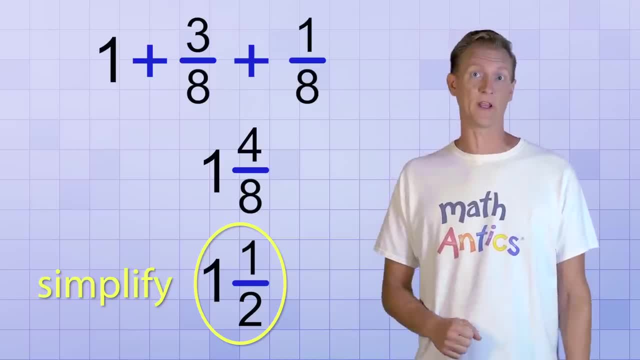 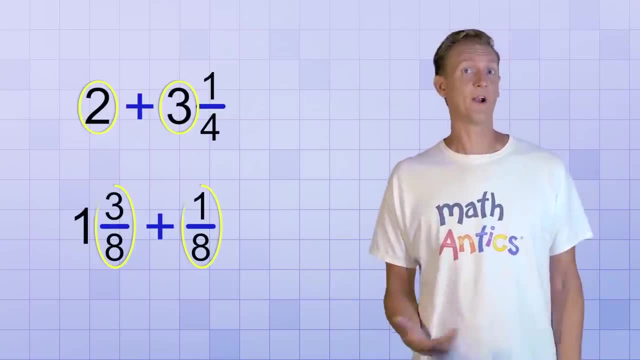 but teachers and tests usually require you to simplify whenever you can, so it's a good habit to get into. Notice that in each of those examples, we just added whole numbers to whole numbers and fractions to fractions, And it works the same way when adding a mixed number to a mixed number. 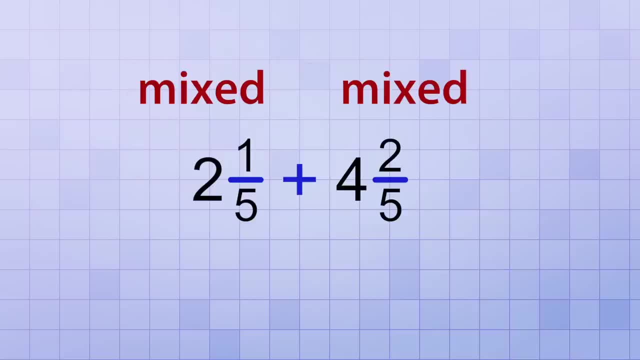 like 2 and 1 fifth plus 4 and 2 fifths. Again, let's show our mixed numbers with the plus signs so we can see the real problem: 2 plus 1 fifth plus 4 plus 2 fifths. 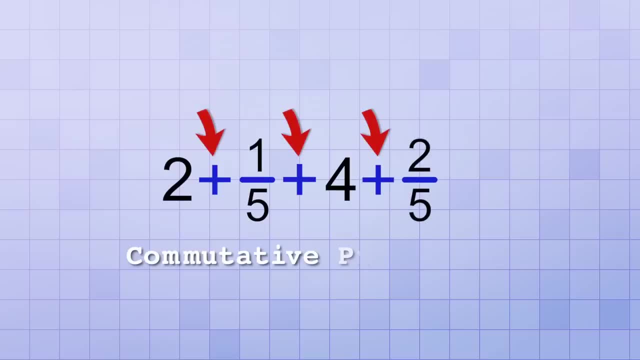 Because all of these parts are being added and addition has the commutative property. it really doesn't matter what order we do. the addition in. That means we can rearrange it. We can change this problem to make it simpler. Now we have 2 plus 4 plus 1 fifth plus 2 fifths. 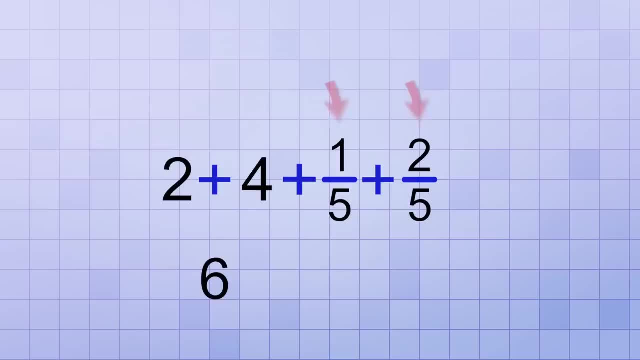 Adding the whole numbers is easy: 2 plus 4 equals 6.. And adding these like fractions is easy too: 1 fifth plus 2 fifths equals 3 fifths. That leaves us with 6 plus 3 fifths, which is the mixed number 6 and 3 fifths. 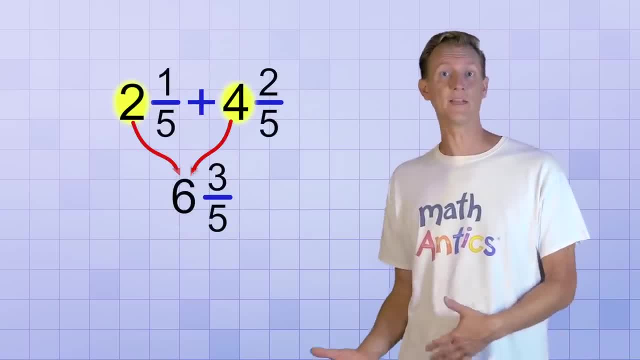 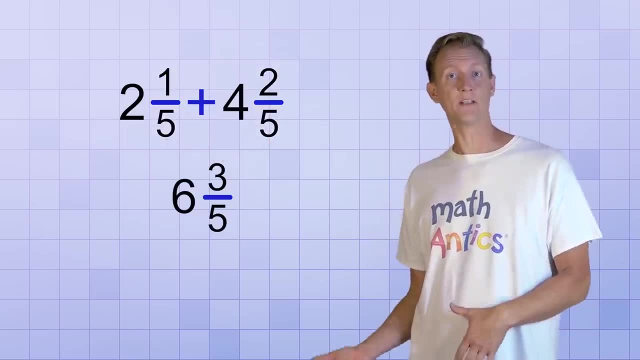 So when you add mixed numbers you can just add the whole number parts to get the whole number of the answer And you add the fraction parts to get the fraction part of the answer. That's why in a lot of math books you'll see the addition of mixed numbers written in a stacked form like this: 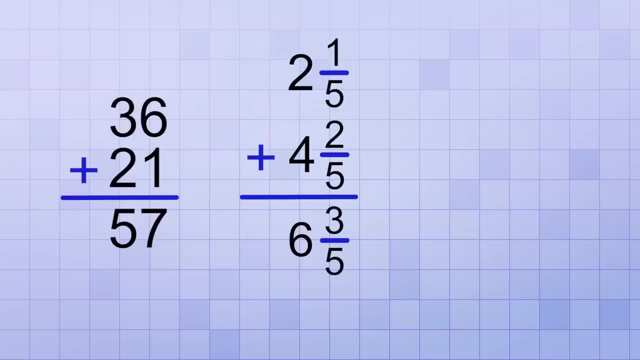 This is similar to the way you would stack multi-digit numbers up to add them, And it helps you remember that you can add the fraction parts and the whole number parts in two separate columns and write your answer below the answer line, just like in multi-digit addition. 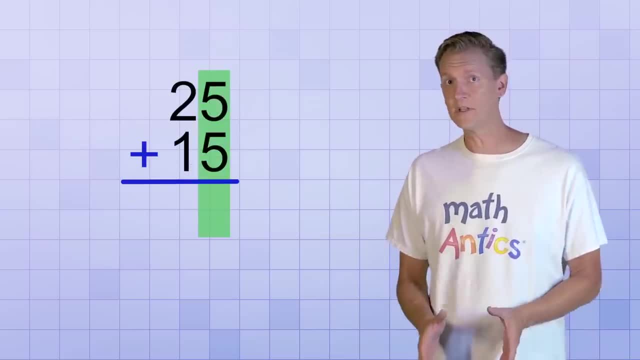 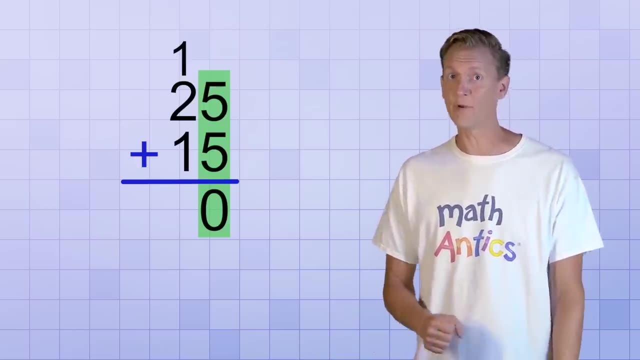 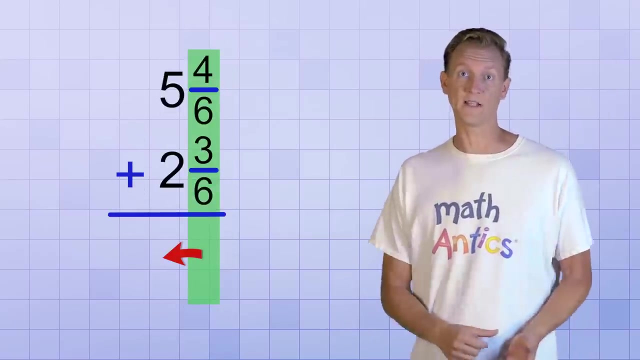 And do you remember how, in multi-digit addition, if a column of digits added up to 10 or more, you had to carry or regroup to the next column? Well, something similar to that can happen when adding mixed numbers. Sometimes adding the fraction parts of two mixed numbers actually affects the whole number. part of the answer. 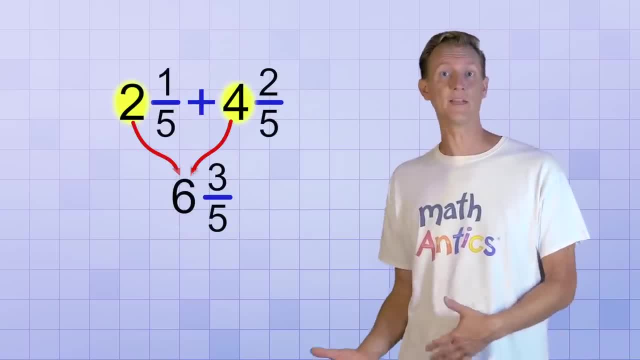 So when you add mixed numbers, you can just add the whole number parts to get the whole number of the answer. And you add the fraction parts to get the fraction part of the answer. 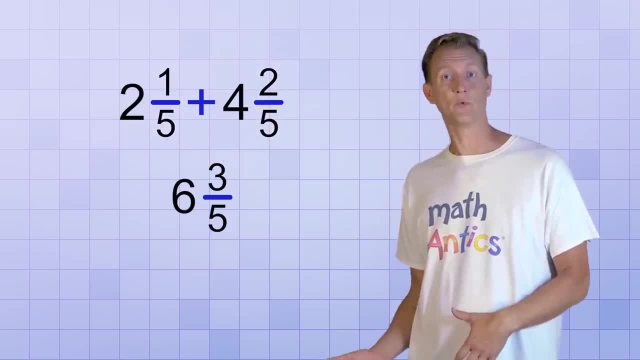 That's why in a lot of math books, you'll see the addition of mixed numbers written in a stacked form like this. 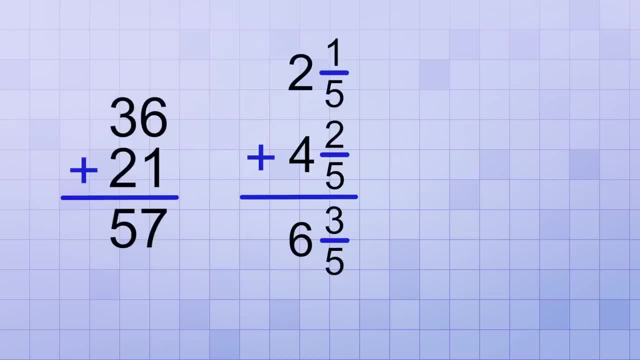 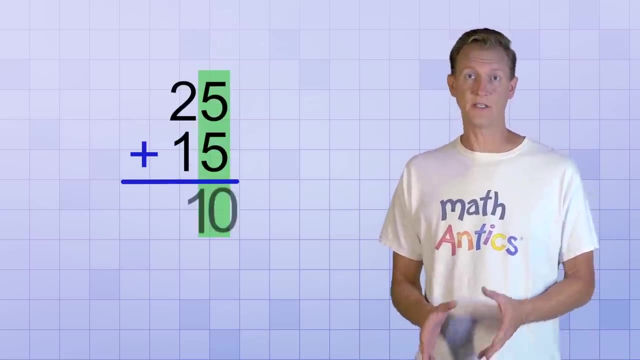 This is similar to the way you would stack multi-digit numbers up to add them. And it helps you remember that you can add the fraction parts and the whole number parts in two separate columns and write your answer below the answer line just like in multi-digit addition. And do you remember how in multi-digit addition, if a column of digits added up to 10 or more, you had to carry or regroup to the next column? Well, something similar to that can happen when adding mixed numbers. 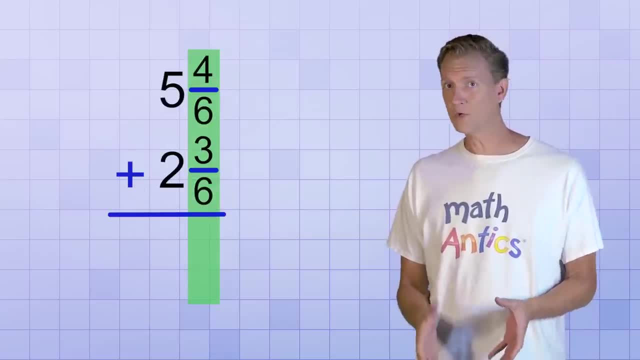 Sometimes, adding the fraction parts of two mixed numbers actually affects the whole number part of the answer. 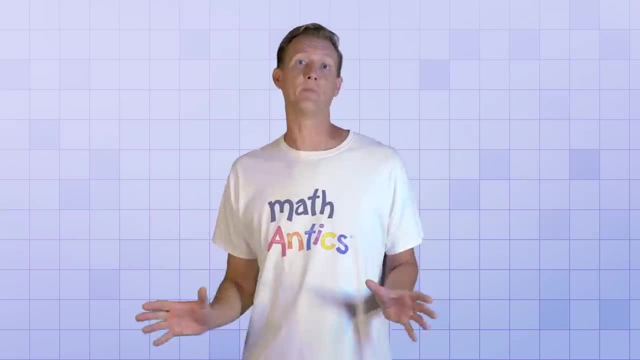 To see what I mean by that, let's say you hosted a massive pizza party for all your friends. Hey man, this is a great party! We got some really cool friends! 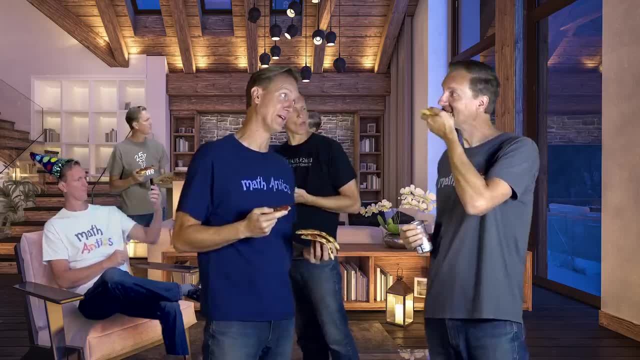 Hey, thanks! You should hang out with us more often. I think you'd really fit in. 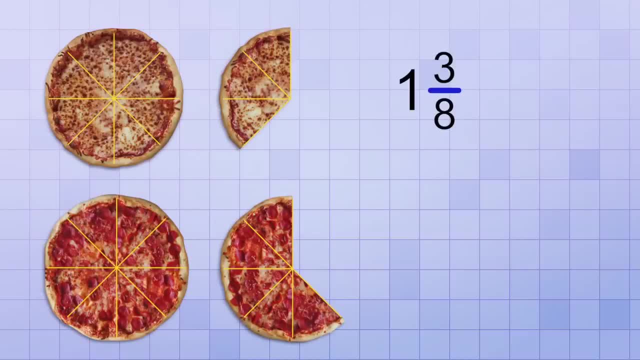 And after the party ended, you had 1 and 3 eighths cheese pizzas left over and 1 and 5 eighths pepperoni pizzas left over. 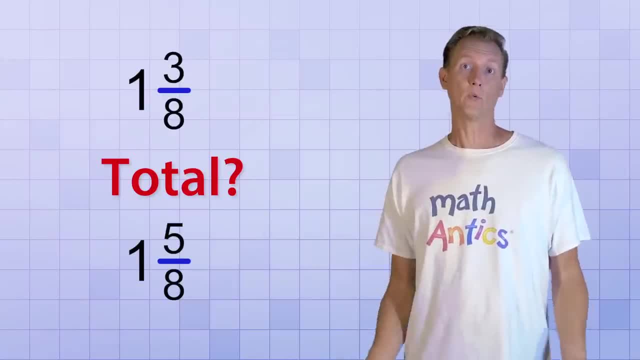 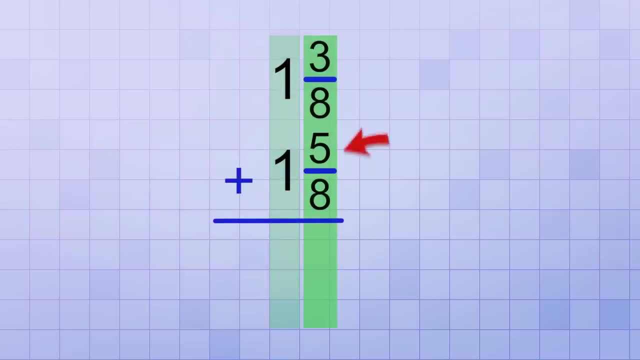 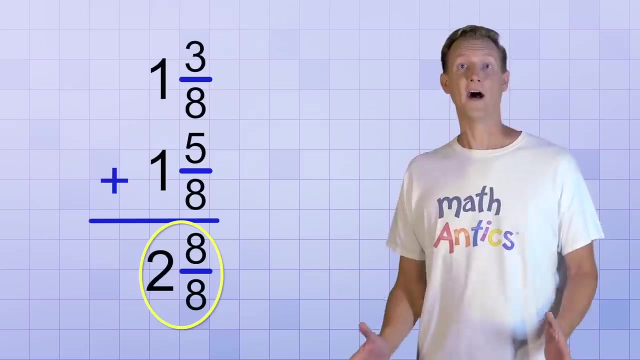 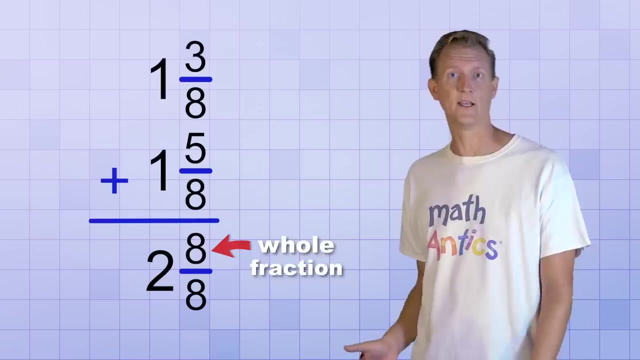 What's the total amount of leftover pizza? Well, we just need to add those two mixed numbers together. Let's stack them like I just showed you and add them column by column. 3 eighths plus 5 eighths equals 8 eighths. And 1 plus 1 equals 2. So the answer is 2 and 8 eighths. Ah, but do you see what happened? The fraction parts of the two mixed numbers combine to form what I call a whole fraction, 8 over 8. 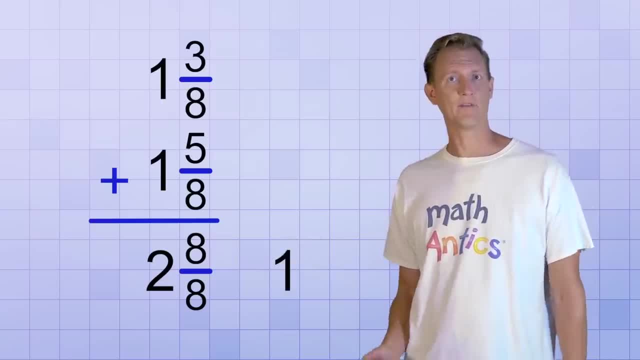 And we know that 8 over 8 simplifies to 1. So having 2 plus 8 over 8, is the same as having 2 plus 1, which is 3. 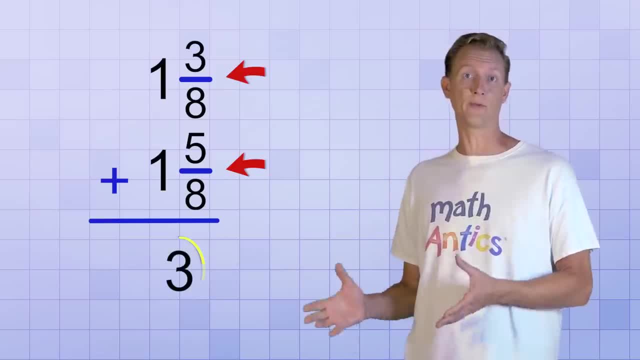 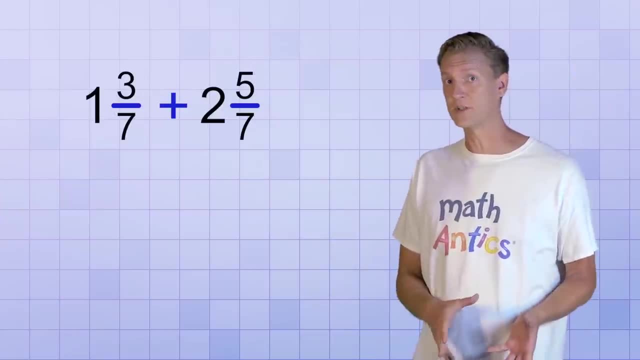 We added two mixed numbers together and ended up with the whole number 3. And our leftover pizza shows us that we got the answer right. Here's another example that shows how the fraction parts 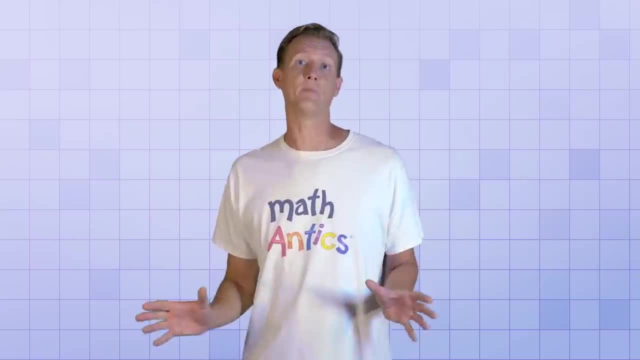 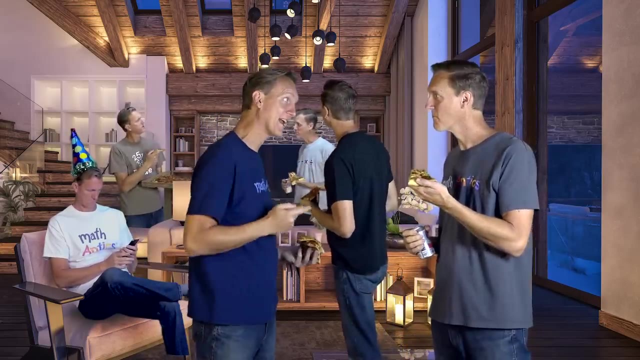 To see what I mean by that. let's say, you hosted a massive pizza party for all your friends. Hey man, this is a great party. We got some really cool friends. Hey, thanks, You should hang out with us more often. I think you'd really fit in. 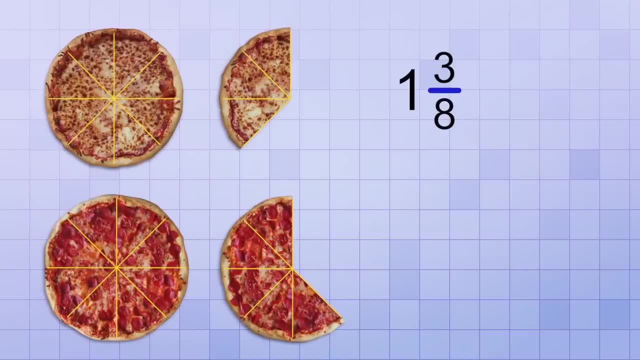 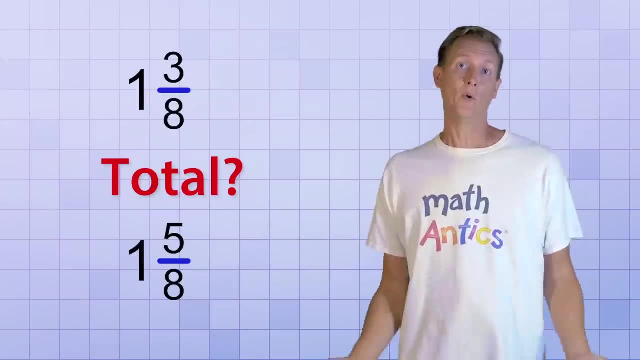 And after the party ended, you had 1 and 3 eighths cheese pizzas left over and 1 and 5 eighths pepperoni pizzas left over. What's the total amount of leftover pizza? Well, we just need to add those two mixed numbers together. 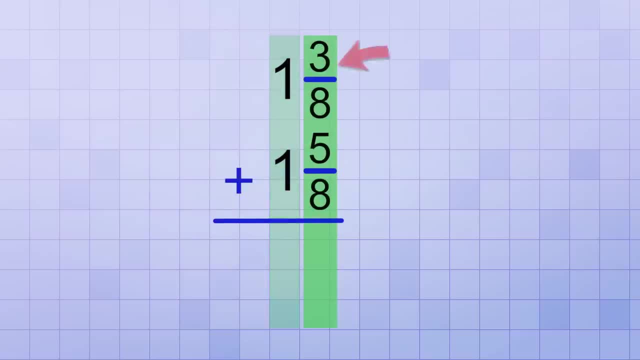 Let's stack them like I just showed you and add them column by column: 3 eighths plus 5 eighths equals 8 eighths, And 1 plus 1 equals 2.. So the answer is 2 and 8 eighths. 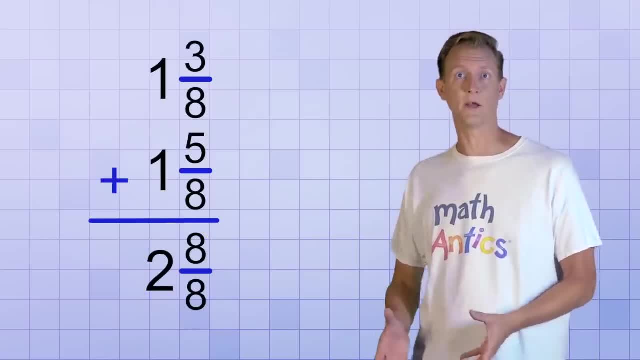 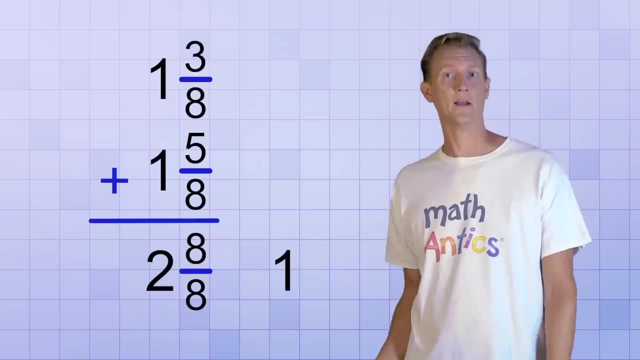 Ah, but do you see what happened? The fraction parts of the two mixed numbers combine to form what I call a whole fraction, 8 over 8.. And we know that 8 over 8 simplifies to 1.. So having 2 plus 8 over 8,. 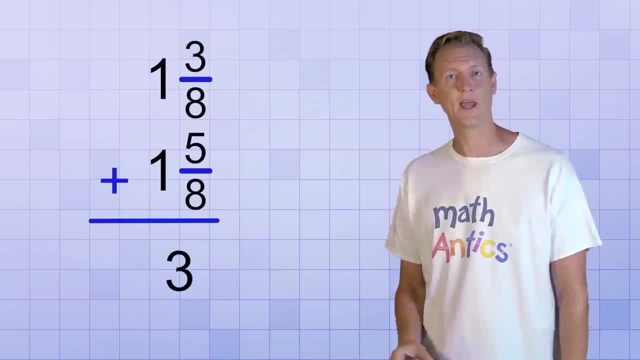 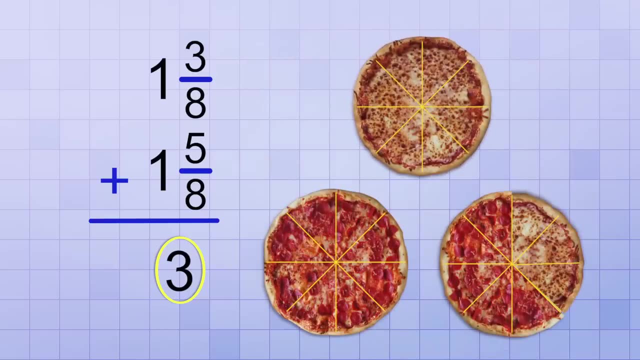 is the same as having 2 plus 1,, which is 3.. We added two mixed numbers together and ended up with the whole number 3.. And our leftover pizza shows us that we got the answer right. Here's another example that shows how the fraction parts. 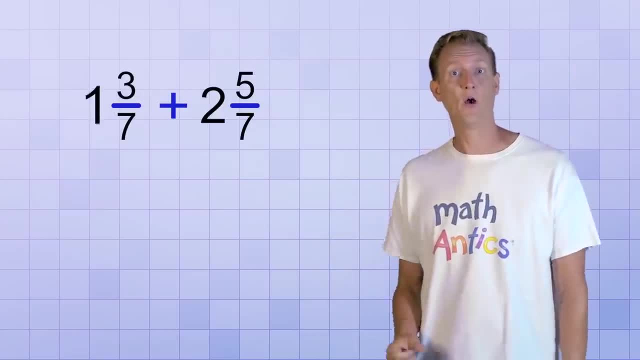 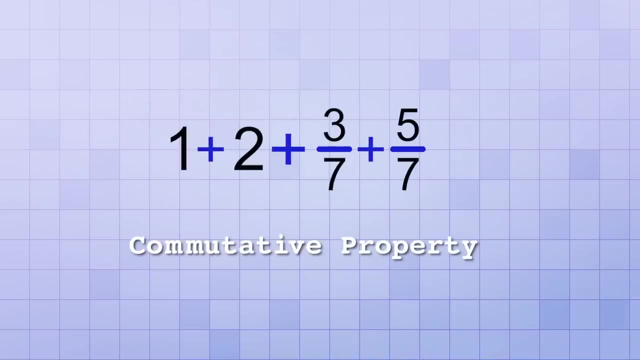 can affect the whole number. part of the answer when adding mixed numbers- 1 and 3 sevenths plus 2 and 5 sevenths. This time we'll use the commutative property to rearrange the addition and then we add the whole number. parts 1 plus 2 equals 3,. 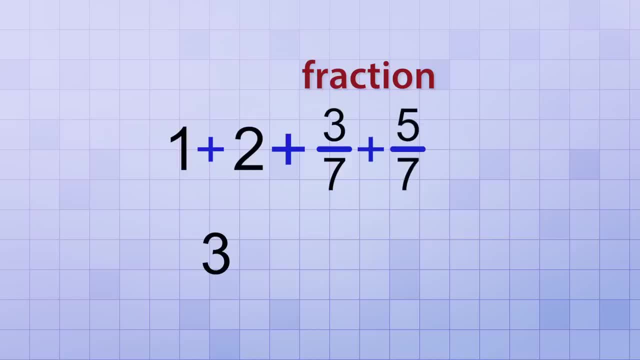 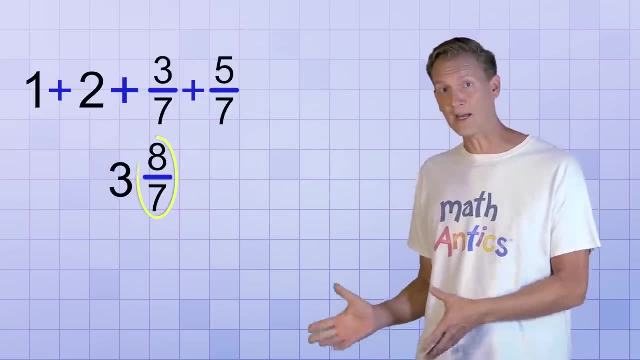 and then we'll add the fraction parts: 7 sevenths plus 5 sevenths equals 8 sevenths. So the answer we get is 3 and 8 sevenths. But do you notice something funny about the fraction part of that answer? 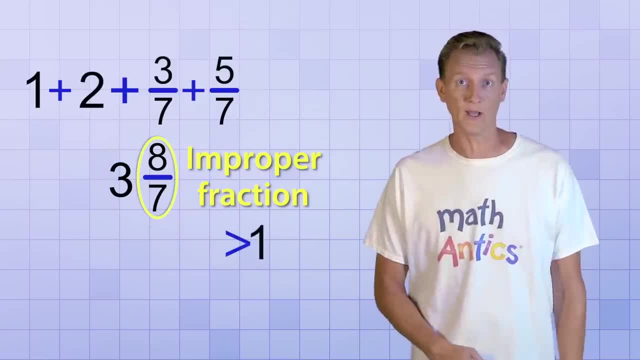 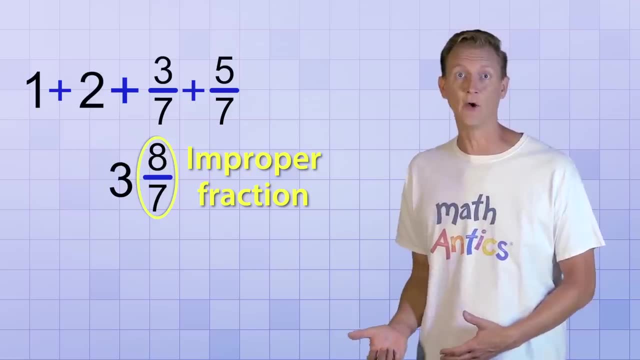 It's an improper fraction, which means that its value is greater than 1.. And it's really bad form to leave an improper fraction in a mixed number like this, because, as we saw in the last video, the improper fraction itself can be converted into a mixed number. 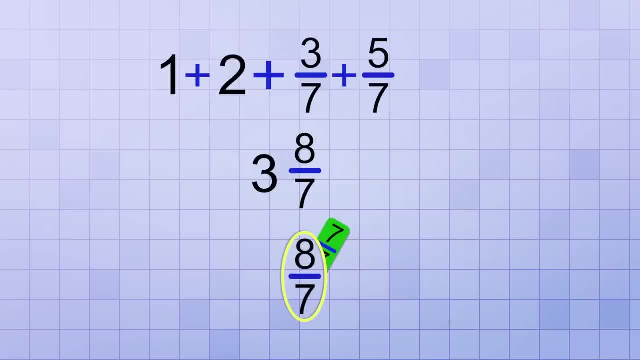 8 over 7 contains a whole fraction that we can simplify out of it. It's the same as 7 over 7 plus 1 over 7.. And since 7 over 7 equals 1, that gives us the mixed number 1 and 1- seventh. 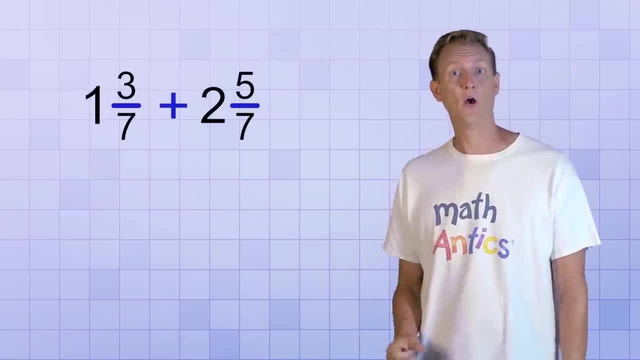 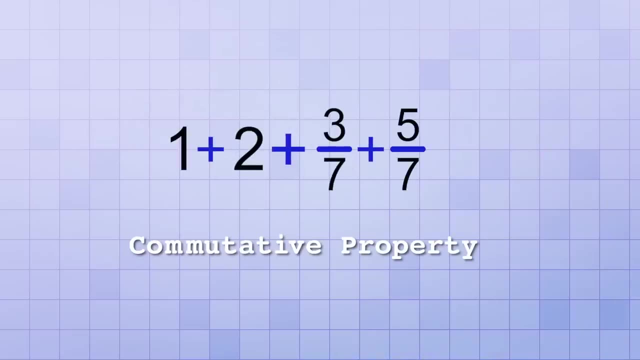 can affect the whole number part of the answer when adding mixed numbers. 1 and 3 sevenths plus 2 and 5 sevenths. This time we'll use the commutative property to rearrange the addition and then we add the whole number parts, 1 plus 2 equals 3, and then we'll add the fraction parts, 7 sevenths plus 5 sevenths equals 8 sevenths. 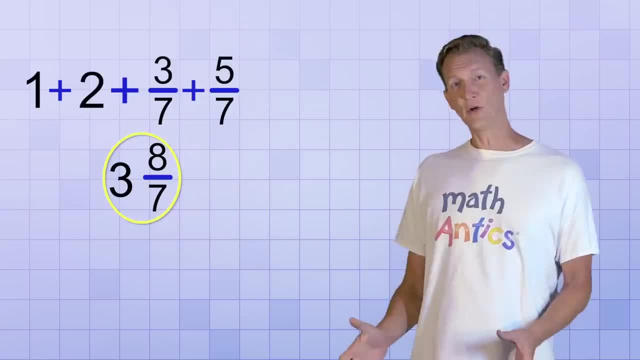 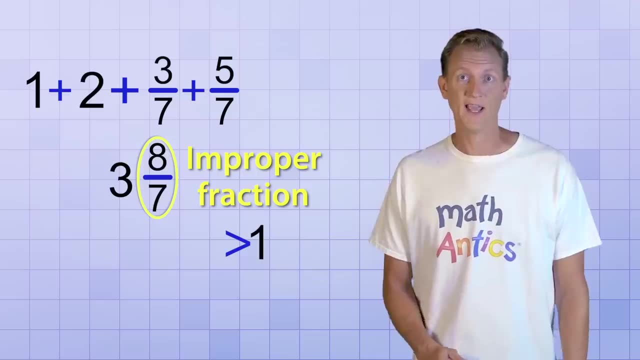 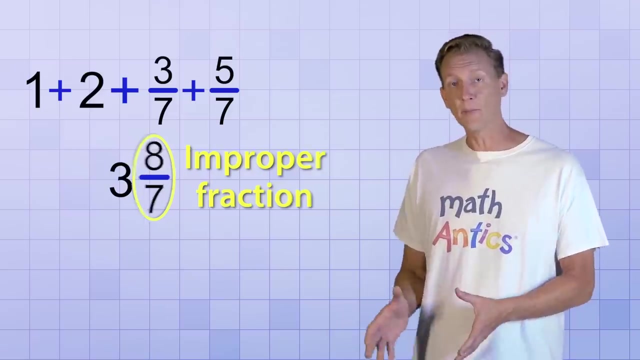 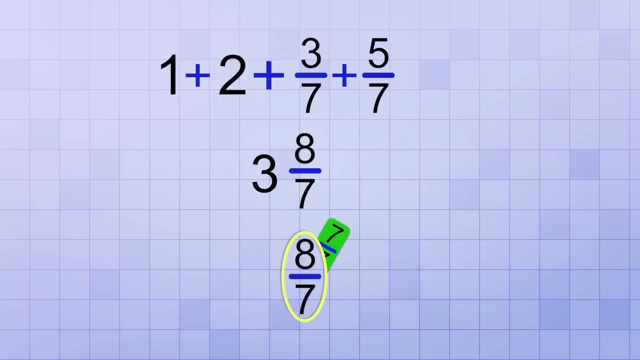 So the answer we get is 3 and 8 sevenths. But do you notice something funny about the fraction part of that answer? It's an improper fraction, which means that its value is greater than 1. And it's really bad form to leave an improper fraction in a mixed number like this, because, as we saw in the last video, the improper fraction itself can be converted into a mixed number. 8 over 7 contains a whole fraction that we can simplify out of it. It's the same as 7 over 7 plus 1 over 7. And since 7 over 7 equals 1, that gives us the mixed number 1 and 1 seventh. So just like in the last example, we can add that extra 1 to the whole number part of our answer, which gives us 4 and 1 seventh. 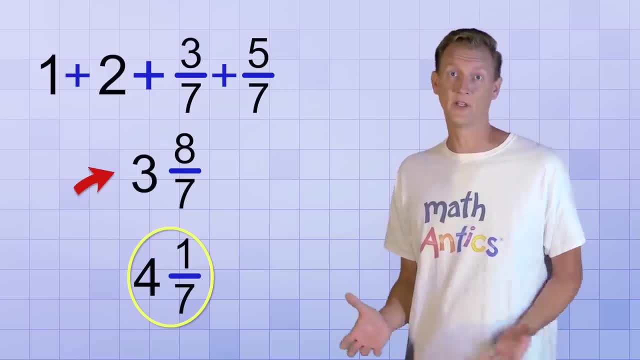 That's a much less confusing answer than 3 and 8 sevenths, which almost sounds like it's less than 4, but it's actually more than 4. Are you getting it so far? 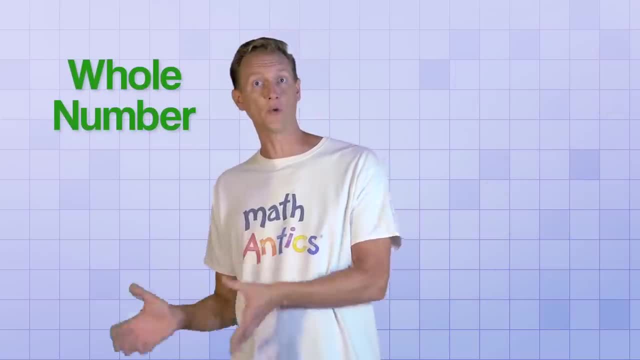 Adding mixed numbers is pretty easy when you realize that you can just add the whole number part of the answer. You can add the whole number parts and the fraction parts separately, and then just watch for cases where the fraction parts add up to more than 1. 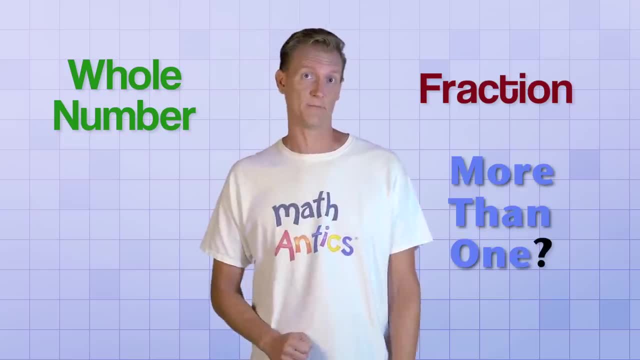 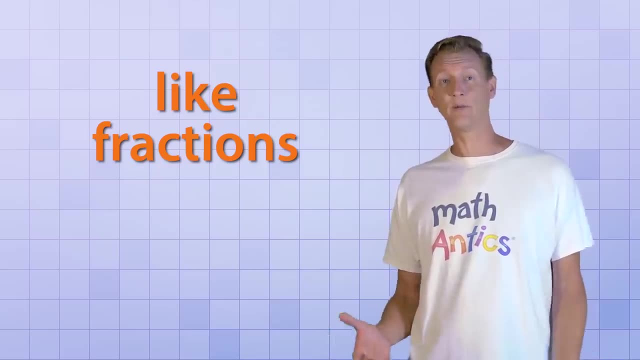 But there are cases where adding mixed numbers can get a little bit tougher. All of the examples we've seen so far had fraction parts that were like fractions. But what if you had to add two mixed numbers with unlike fractions, like this problem? 1 and 1 half plus 2 and 1 fourth. 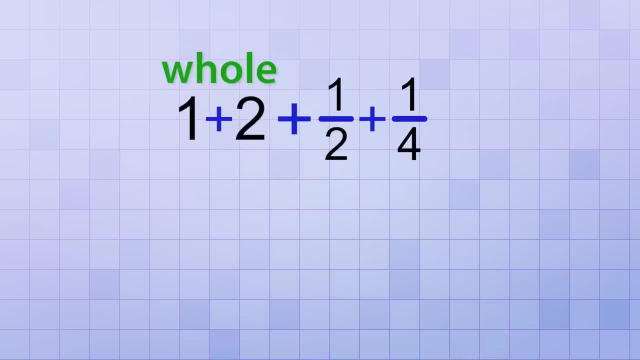 If we rearrange the problem as usual, we see that the whole numbers are still easy to add. 1 plus 2 equals 3. 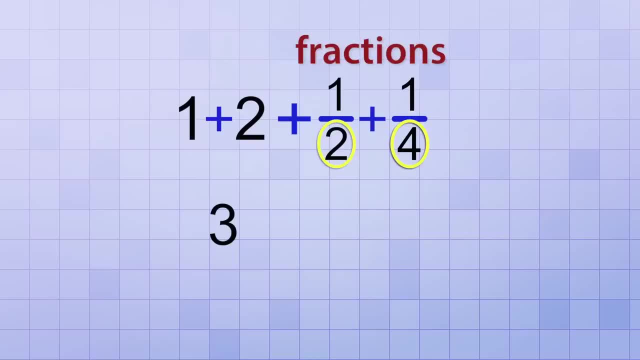 But the fractions have different denominators. We can't add them until we change them so that the bottom numbers are the same. 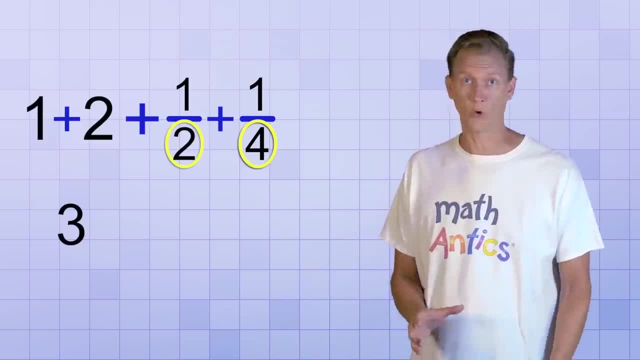 We cover how to change fractions so that they have the same bottom number in other videos that you may want to watch if the steps I'm about to do seem new to you. 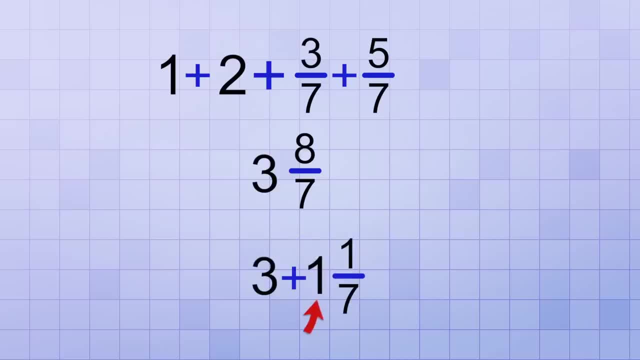 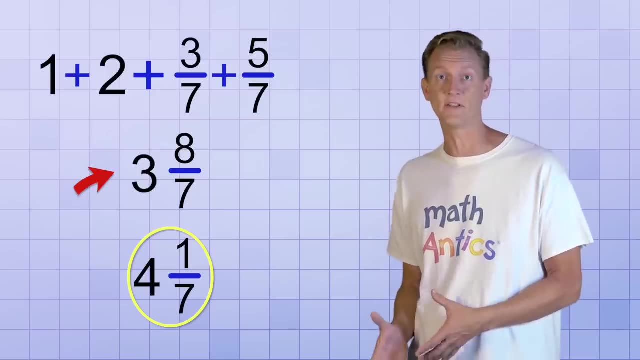 So, just like in the last example, we can add that extra 1 to the whole number part of our answer, which gives us 4 and 1 seventh. That's a much less confusing answer than 3 and 8 sevenths, which almost sounds like it's less than 4, but it's actually more than 4.. 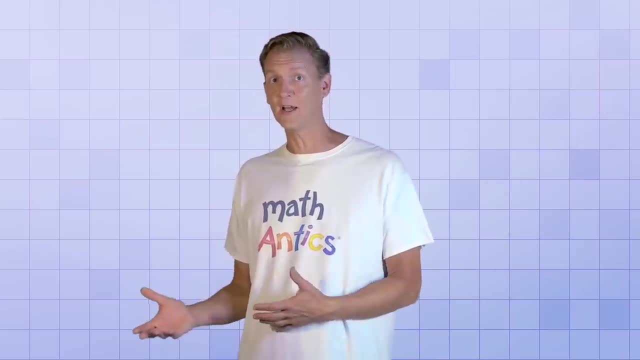 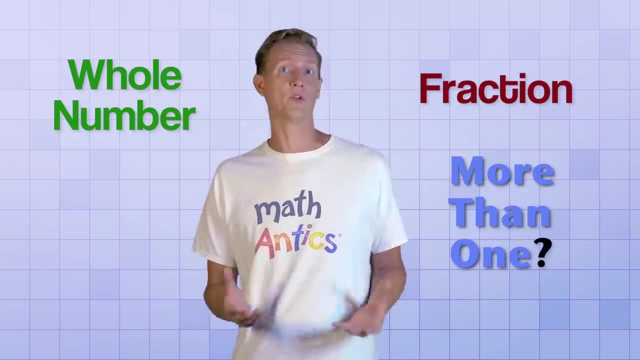 Are you getting it so far? Adding mixed numbers is pretty easy when you realize that you can just add the whole number part of the answer. You can add the whole number parts and the fraction parts separately and then just watch for cases where the fraction parts add up to more than 1.. 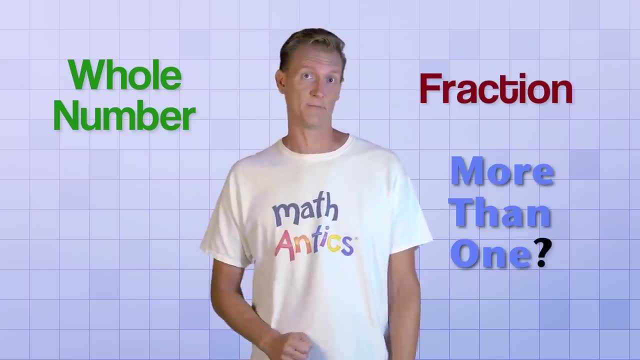 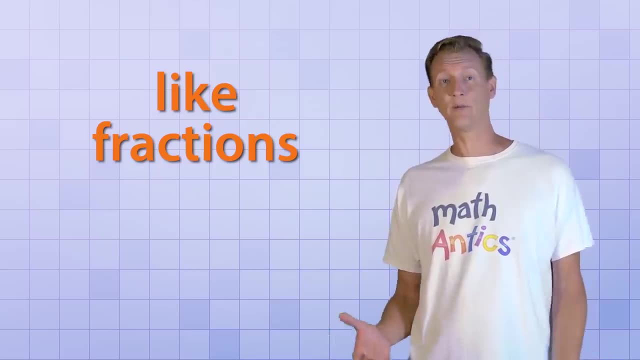 But there are cases where adding mixed numbers can get a little bit tougher. All of the examples we've seen so far had fraction parts that were like fractions. But what if you had to add two mixed numbers with unlike fractions? like this problem: 1 and 1 half plus 2 and 1. fourth, 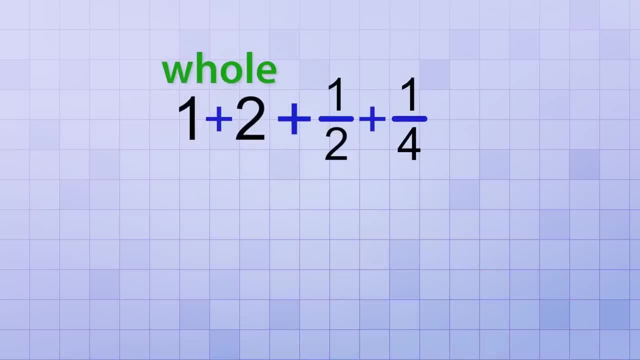 If we rearrange the problem as usual, we see that the whole numbers are still easy to add: 1 plus 2 equals 3.. But the fractions have different denominators. We can't add them until we change them so that the bottom numbers are the same. 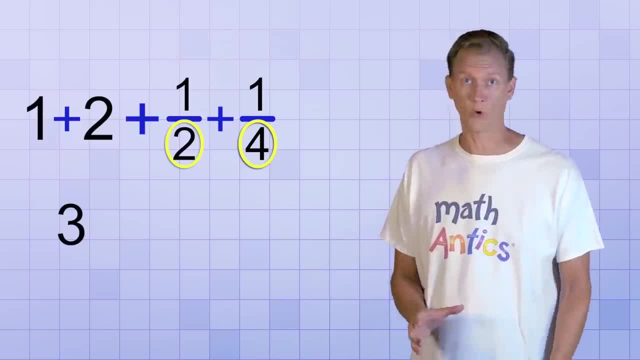 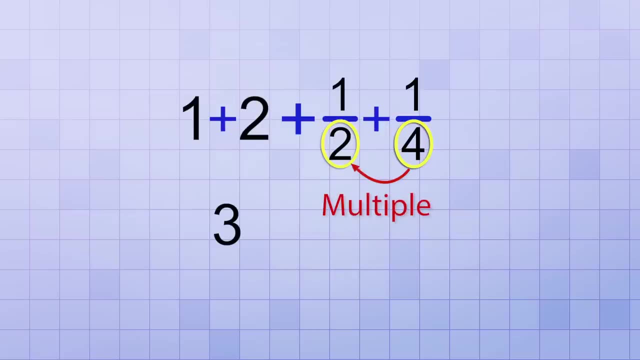 We cover how to change fractions so that they have the same bottom number in other videos that you may want to watch if the steps I'm about to do seem new to you. 4 is a multiple of 2, so 4 is going to be a good choice for a common denominator. 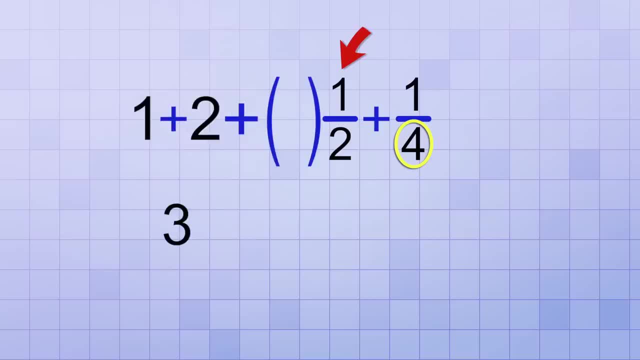 To change 1 half into fourths, we'll multiply it by the whole fraction 2 over 2.. On the top, we have 1 times 2,, which is 2,, and on the bottom we have 2 times 2,, which is 4,, just like we want. 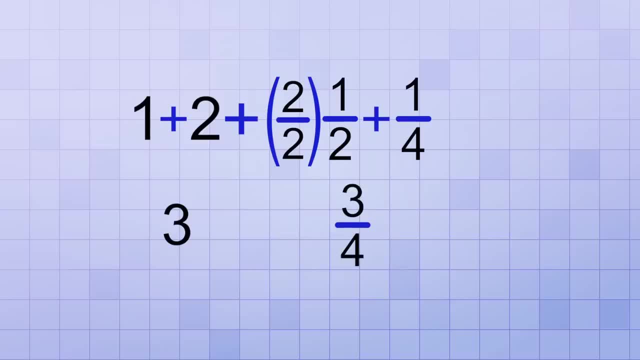 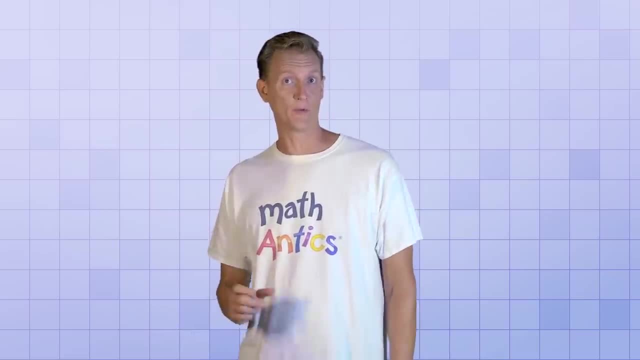 So now we have 2 fourths plus 1 fourth, which equals 3 fourths. That means the answer to this problem is 3 and 3 fourths. That wasn't so bad after all. Let's try one more example where we need to change unlike fractions into like fractions in order to add the mixed numbers. 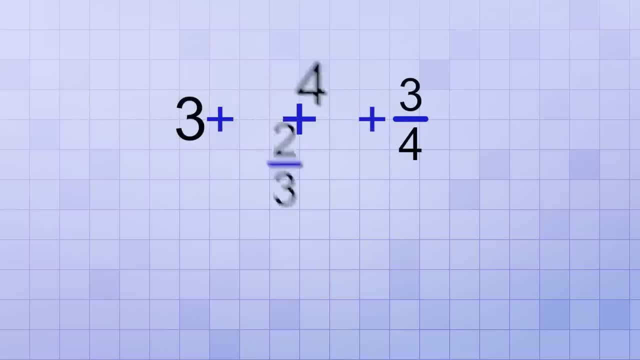 3 and 2 thirds, plus 4 and 3 fourths. After rearranging the parts, we see that we need to add 3 and 4, which is 7, and we also need to add 2 thirds and 3 fourths. 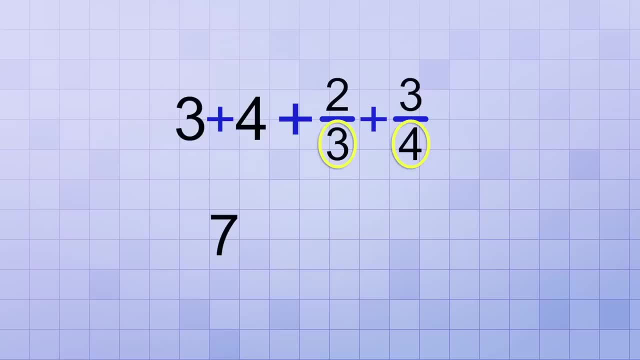 Since these are unlike fractions, we need to change them. 3 and 4 are not multiples of each other, so it looks like using the easiest common denominator will be our best option here. 3 times 4 equals 12, so that will be our new denominator. 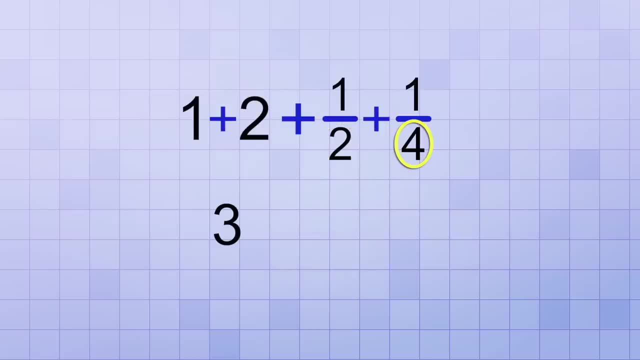 4 is a multiple of 2, so 4 is going to be a good choice for a common denominator. To change 1 half into fourths, we'll multiply it by the whole fraction 2 over 2. On the top, we have 1 times 2, which is 2, and on the bottom, we have 2 times 2, which is 4, just like we want. 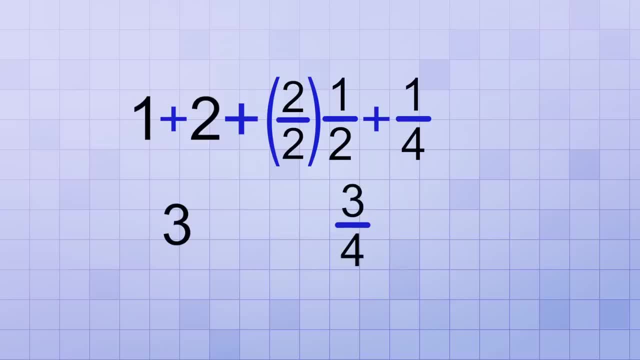 So now we have 2 fourths plus 1 fourth, which equals 3 fourths. That means the answer to this problem is 3 and 3 fourths. That wasn't so bad after all! 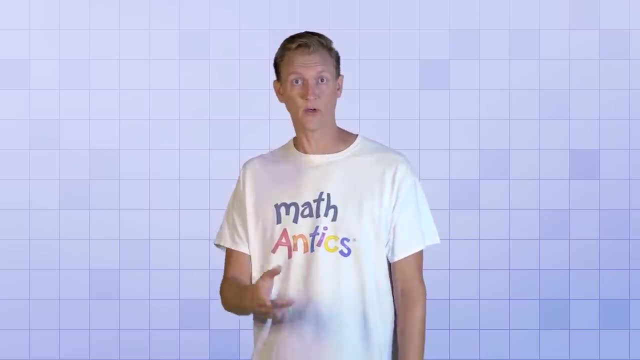 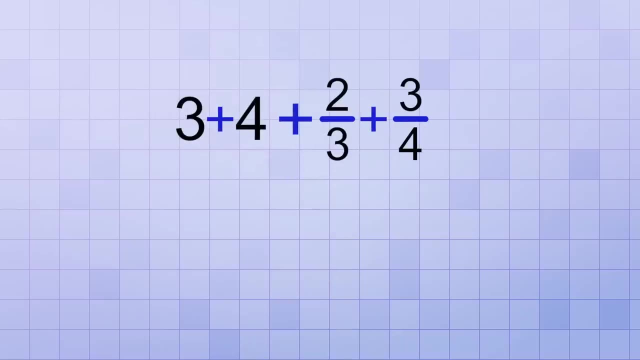 Let's try one more example where we need to change unlike fractions into like fractions in order to add the mixed numbers. 3 and 2 thirds plus 4 and 3 fourths. After rearranging the parts, we see that we need to add 3 and 4, which is 7, and we also need to add 2 thirds and 3 fourths. Since these are unlike fractions, we need to change them. 3 and 4 are not multiples of each other, so it looks like using the easiest common denominator will be our best option here. 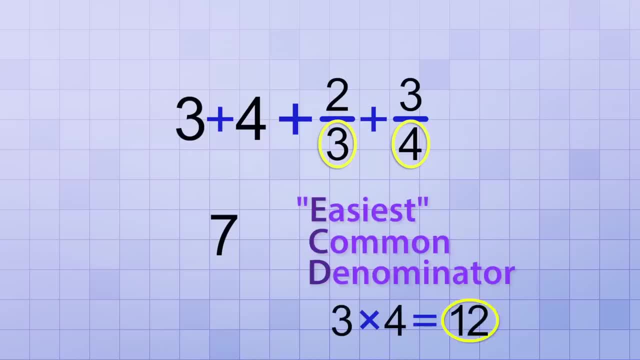 3 times 4 equals 12, so that will be our new denominator. 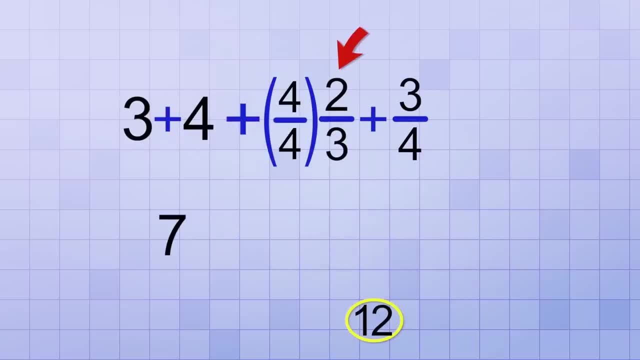 To convert 2 thirds, we multiply it by 4 over 4, which gives us the new equivalent fraction 8 over 12. And to convert 3 fourths, we need to multiply it by 3 over 3, which gives us the new equivalent fraction 9 over 12. Now that we have like fractions, we can add them easily. 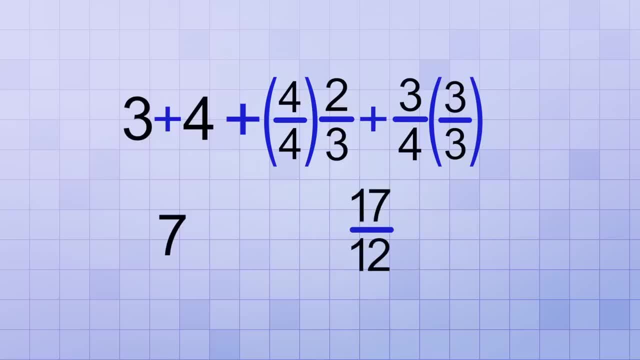 8 over 12 plus 9 over 12 equals 17 over 12. And that gives us 7 and 17 twelfths as our answer. 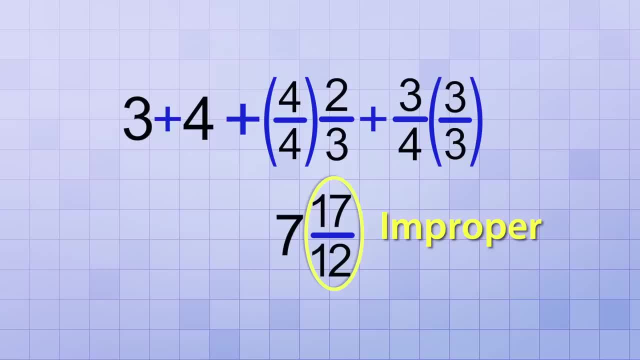 But, once again, the fraction part is improper, so we have to simplify it because its value is greater than 1. 17 over 12 is the same as 12 over 12 plus 5 over 12, which is the mixed number 1 and 5 twelfths. 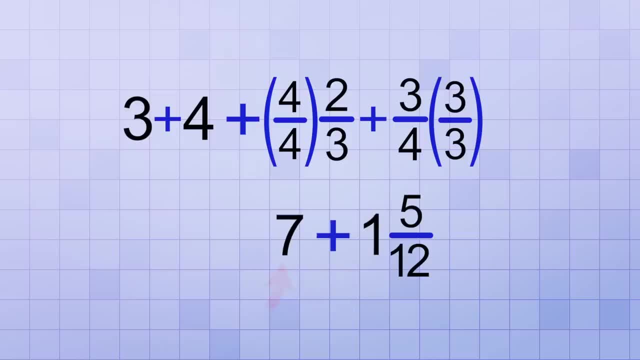 We need to add that 1 to our whole number part. 7 plus 1 equals 8, which means our final answer is… 8 and 5 twelfths.